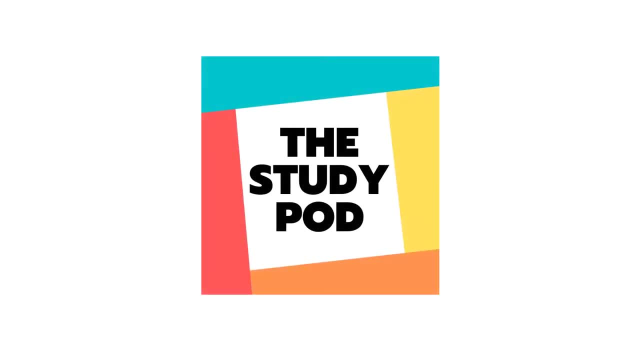 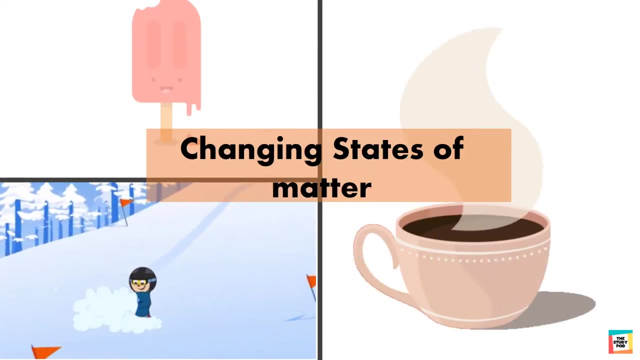 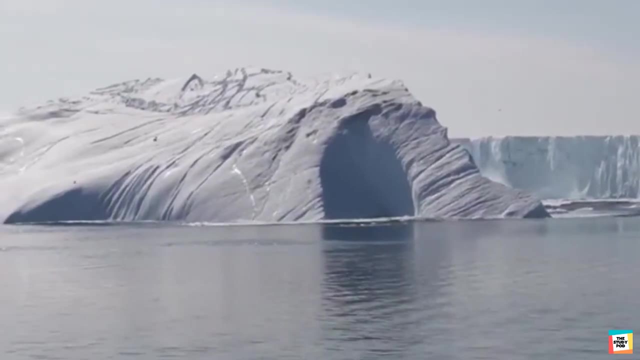 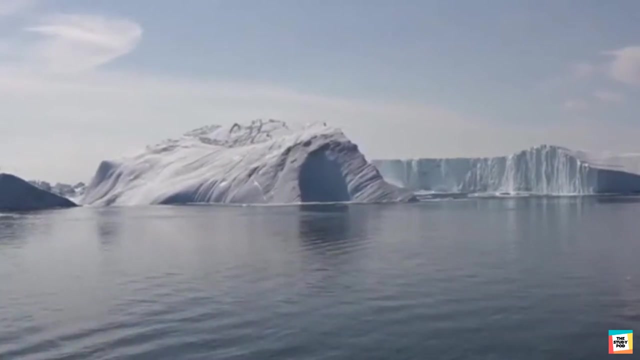 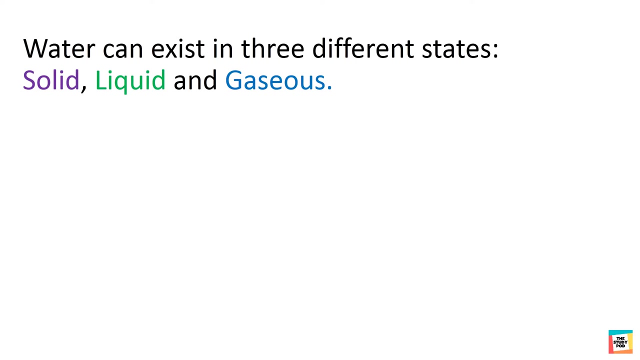 Welcome back, kids. Today we will talk about the changing states of matter. How many states of water you can see in the picture. We can see the liquid water. We can see ice in the form of glaciers. Water is also present in air. in gaseous form, Water can exist in three different states: Solid, liquid and gaseous. 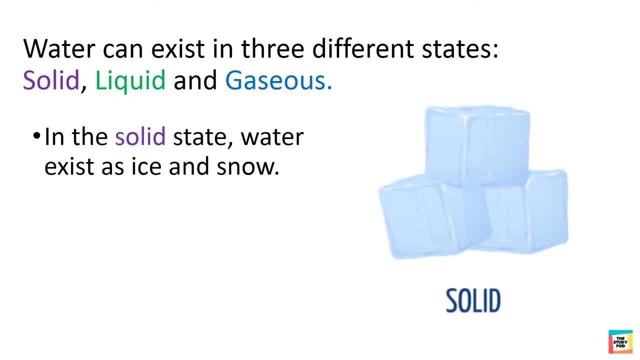 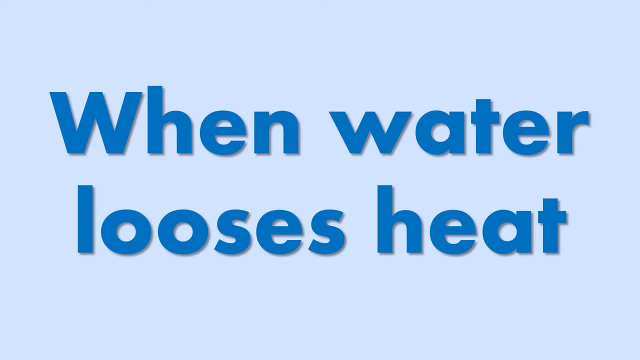 In the solid state, water exists as ice and snow. In liquid state, it exists as liquid water. In gaseous state, it exists as water, vapor or steam. Where do we find ice and snow? How can we change water in the liquid state to water in the solid? 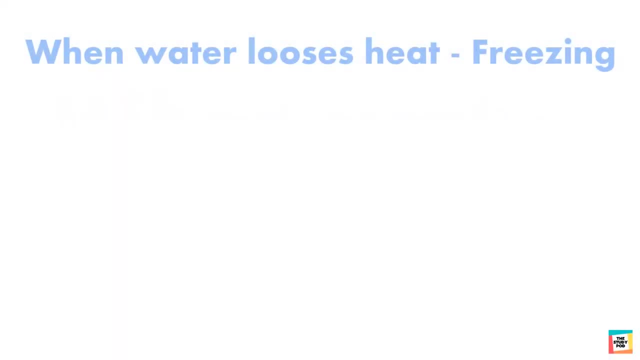 state. Let's find out. When water loses heat, it freezes. Heat flows from a hotter object to a cooler object. Hot object lose heat to their cooler surroundings. When a liquid loses enough heat, it can change into solid. When a liquid changes into solid, we call it freezing The 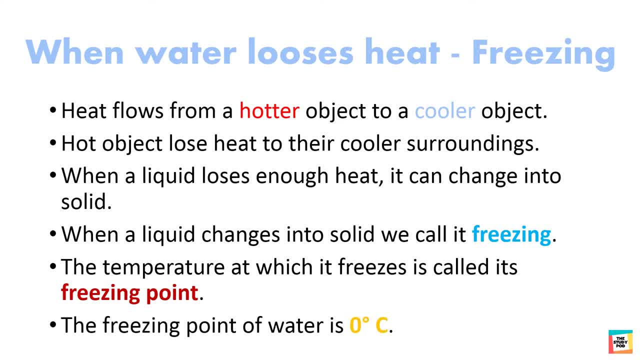 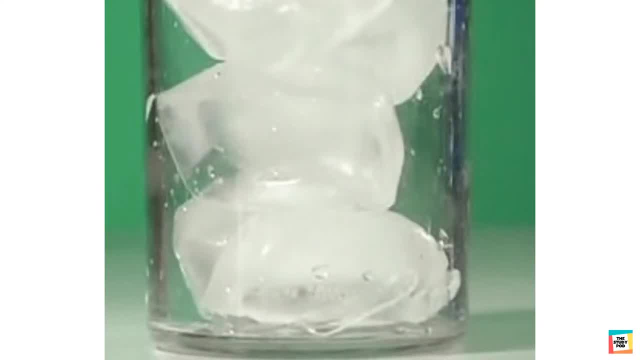 temperature at which it freezes is called its freezing point. The freezing point of water is a zero degree Celsius Пр sue, Fr. whatever. It is cold regardless of temperature. The boiling point of water is the coldest point in the air. When the temperature Silence is less than the temperature, chill in the air takes about. 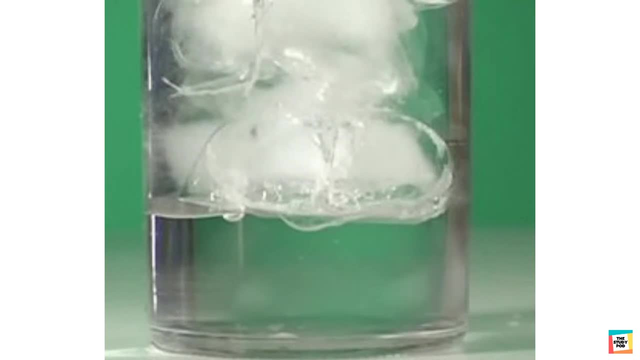 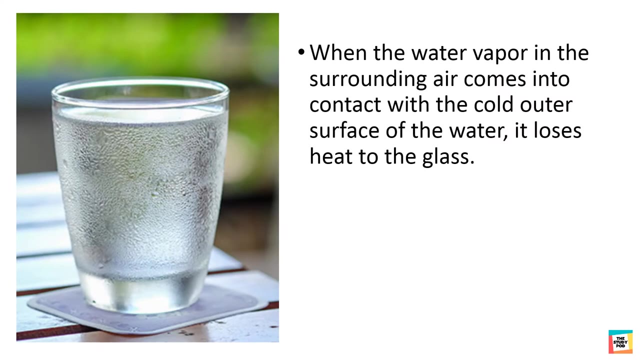 15 minutes and changes to water. This is 100%ат. When the temperature is like this, The temperature that rises and falls in this of when water goes down changes into rocks. The water vapor comes in the coldest part of water. 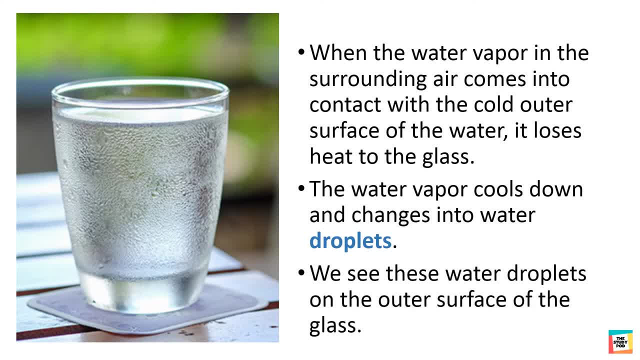 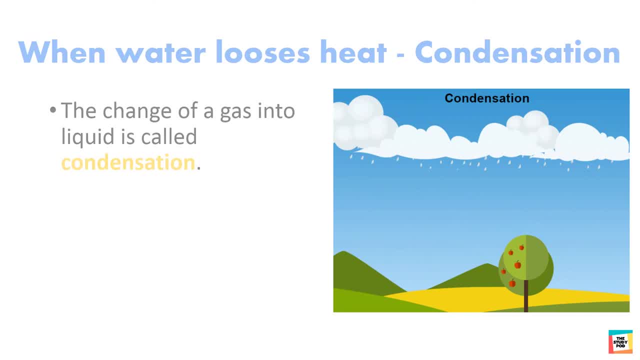 What can be faster than the water temperature? We see these water droplets on the outer surface of the glass. When water loses heat, it condenses. The change of a gas into liquid is called condensation. When water in gaseous state loses enough heat, it condenses into liquid water. 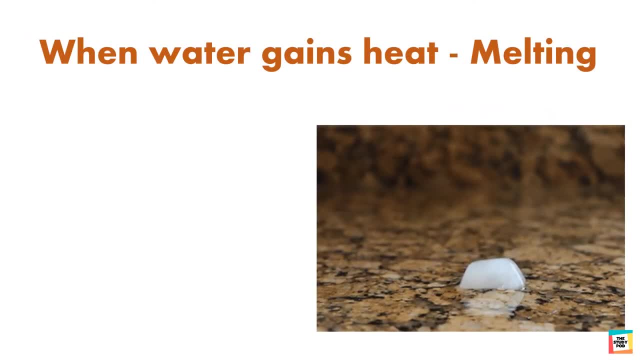 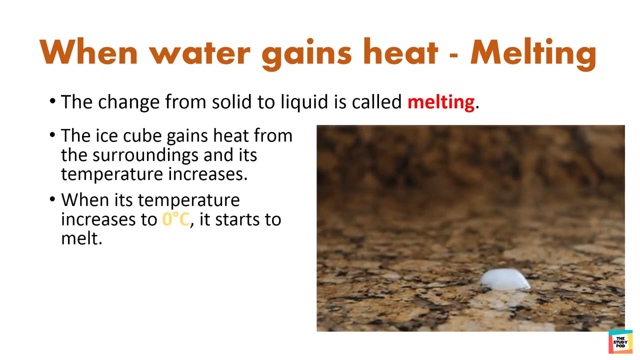 If you leave an ice cube outside the freezer, it changes from solid ice into water after some time. The change from solid to liquid is called melting. The ice cube gains heat from the surroundings and its temperature increases. When its temperature increases to zero degree, it starts to melt. 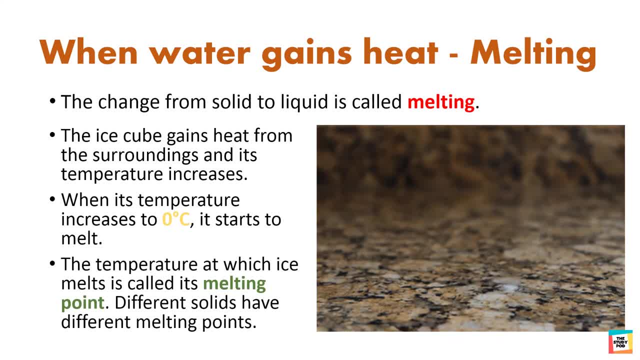 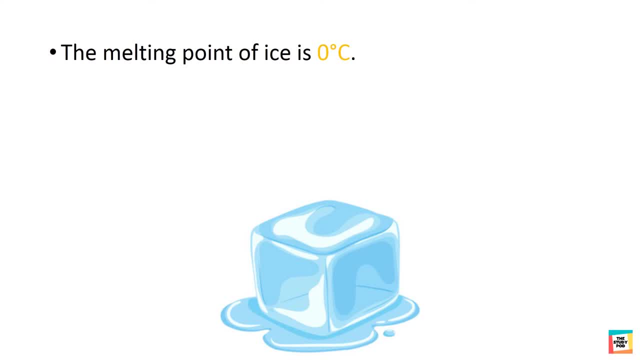 The temperature at which ice melts is called its melting point. Different solids have different melting points. The melting point of ice is zero degrees. The melting ice remains at this temperature until autumn. All of the ice has melted. Do you notice that the melting point of ice is the same as the freezing point of water? 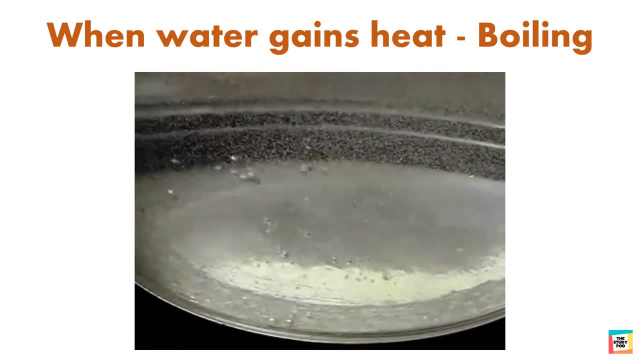 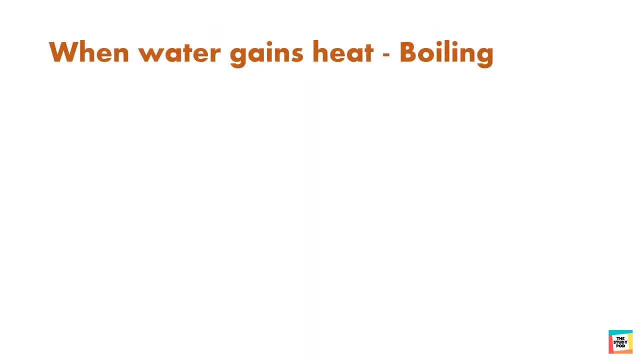 When we boil water, we see bubbles in the boiling water. What do these bubbles contain? The level of liquid water decreases with time. What happens to the water? What causes this change? Let's find out. When water gains heat, it boils. 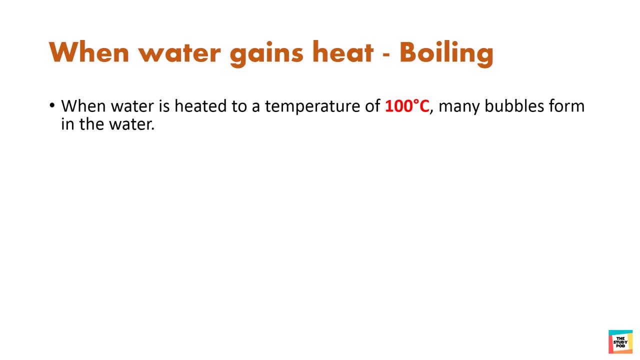 When the water is heated to a temperature of 100 degrees Celsius, many bubbles form in the water. These bubbles contain water in gaseous state. They are formed when the liquid water gains heat and changes into gas. Pure liquid water changes into steam at 100 degrees Celsius. 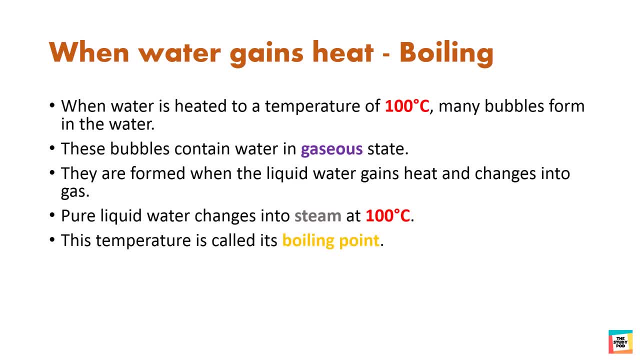 This temperature is called its boiling point. The change of a liquid into a gas at its boiling point is called boiling, Although the temperature of the liquid water changes. the temperature of the liquid water changes. Although the water continues to gain heat during boiling, its temperature does not increase during the process. 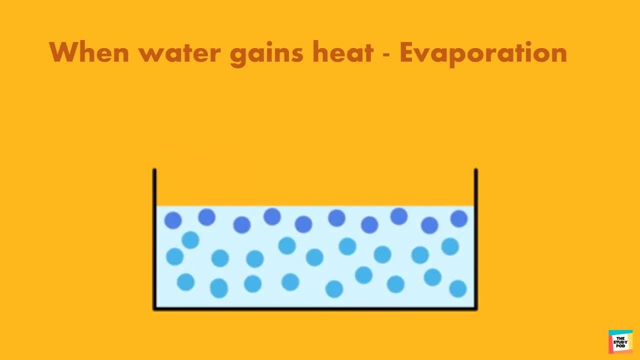 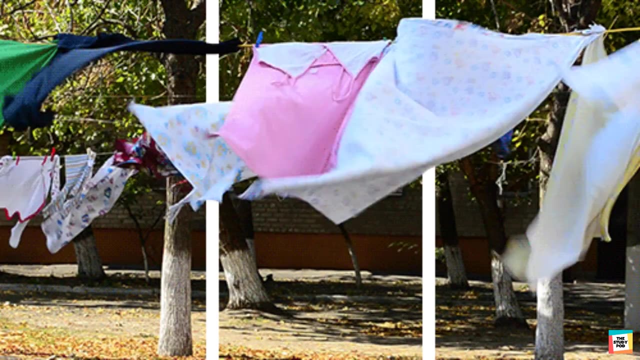 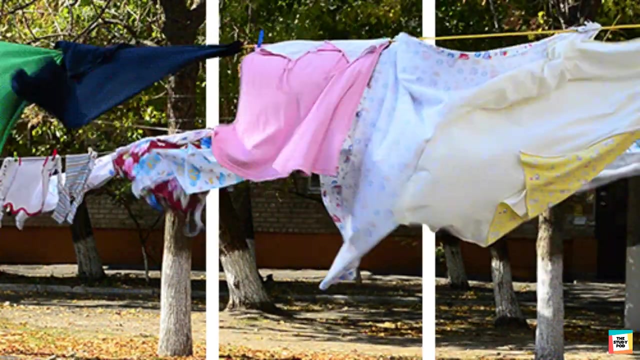 Liquid water can change into gas without boiling too. The change of a liquid into a gas below its boiling point is called evaporation. We hang out clothes to dry. After some time the wet clothes will become dry. The liquid water in the clothes will gain heat from the surroundings and will change into water vapor. 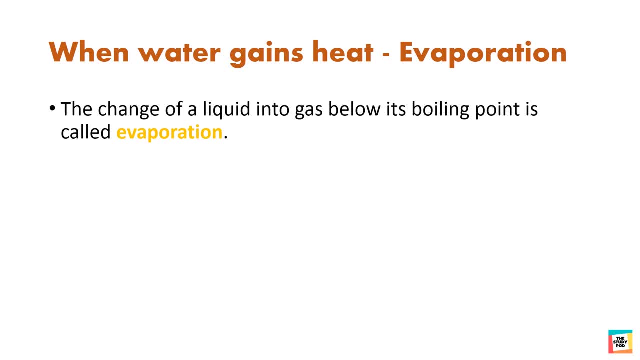 The change of a liquid into a gas below its boiling point is called evaporation. How quickly evaporation takes place is called rate of evaporation. The rate of evaporation depends upon The temperature of the surroundings. Water evaporates quickly in higher temperature. 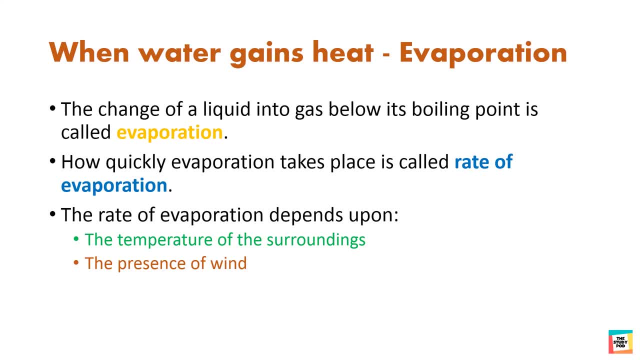 The presence of wind, Water evaporates quickly. in the presence of wind. The surface area Water evaporates quickly. when surface area add more heat, Water will be torn into pieces, followed by vapor and deофether. material is larger humidity, which is the amount of water vapor in the air. water evaporates quickly when 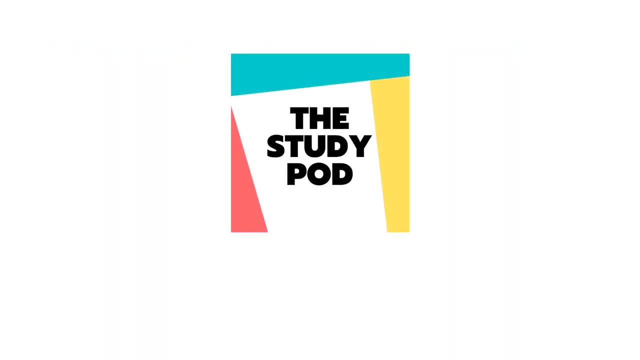 humidity is low. this brings us to the end of the video. if you have any queries, you can write to us.